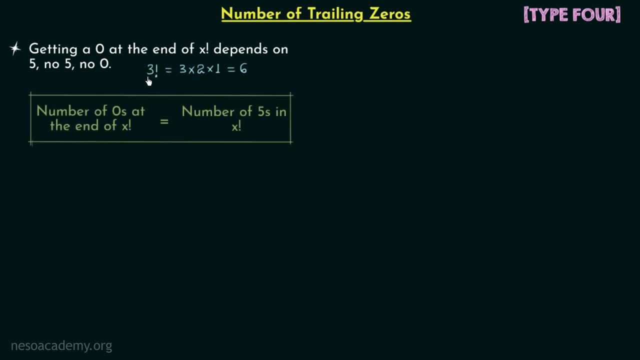 there is no 0 at the end. And with this we can conclude. the number of zeros at the end of x factorial is equal to the number of 5s in the x factorial. And now we will solve few more examples to understand this better. Example 1 is 5 factorial. We know 5 factorial is equal to 5. 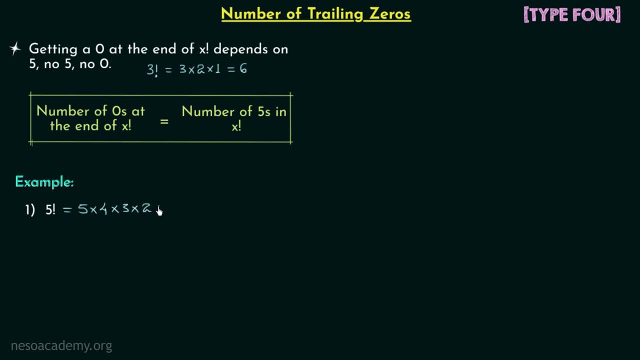 multiplied to 4, multiplied to 3, multiplied to 2, multiplied to 1.. And when you solve this, you will have 120 as the result, And you can clearly see that we have one 0 at the end. There is one trailing zero in the result, And when you solve this, you will have 120 as the result. 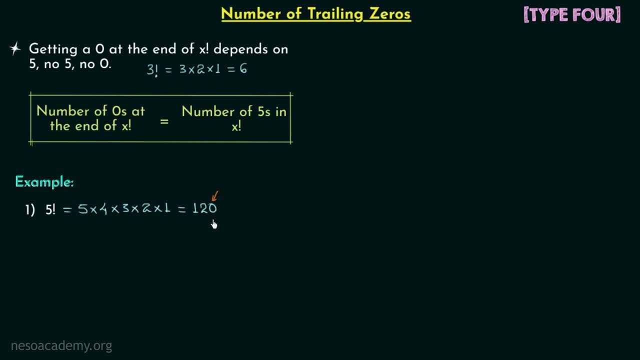 5 factorial And this one 0, we are getting because we have one 5 present in the expansion. Now the question is: why do we get 0 at the end whenever we have 5 in the expansion? And the answer is: 5 when multiplied to an even number produces a number having 0 at the end, 5 here. 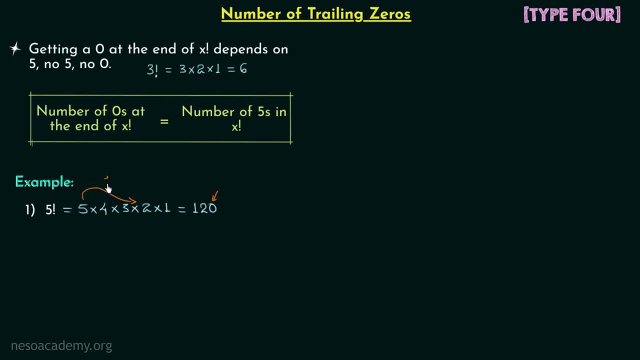 when multiplied to 2 will produce 10.. And here you can see we have 0 at the end. So single 5 in the expansion gave us single 0 at the end. Now let's see the example number 2.. We have 10 factorial And we know 10 factorial is equal to 10. 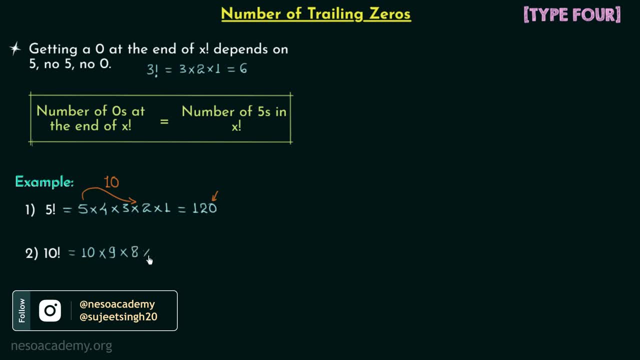 multiplied to 9. multiplied to 8. multiplied to 7. multiplied to 6. multiplied to 5. multiplied to 4. multiplied to 12. multiplied to 1. multiplied to 7. multiplied to 9. multiplied to 8. multiplied to 9. multiplied to 9. 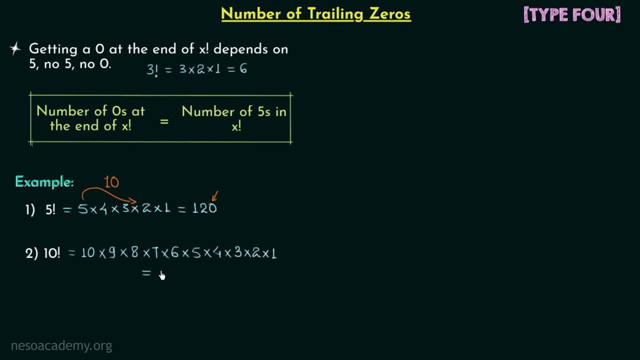 multiplied to 10, to 3, multiplied to 2, multiplied to 2, multiplied to 1, and then multiplied to 1.. And when you solve this you will have 3628800.. So in this way we are getting two zeros at the end of 10 factorial, And the reason is presents of: 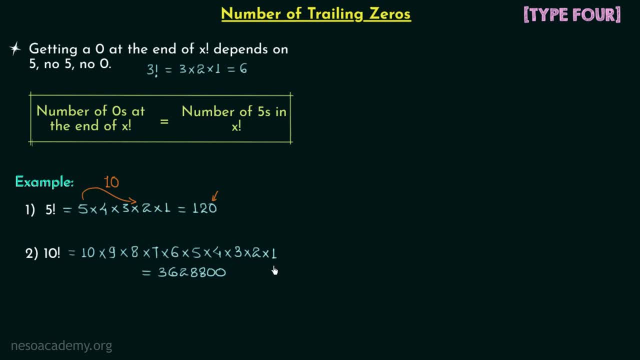 two five's in the expansion. let us find out the two fives in this expansion. The first five is clearly visible And the second is created in the first path at the end. So we'll called it 2: 0. And the reason is: presence of the two 5s is in the level of 4.. So with this value of 10, then we are required of 5 and a half, then 1 plus 2. 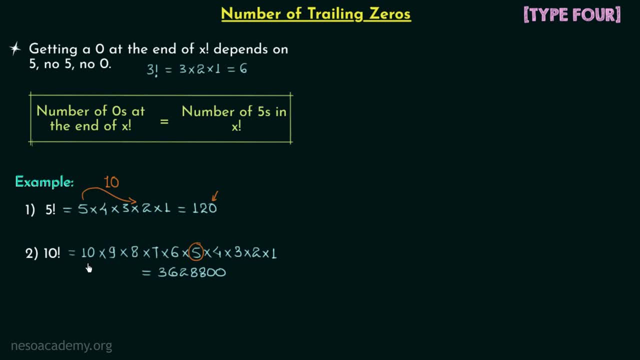 and the second 5 can be obtained from 10.. 10 is equal to 5 multiplied to 2. So our second 5 is in this 10.. So total two 5s are there in the expansion and hence we have two 0s at the end. 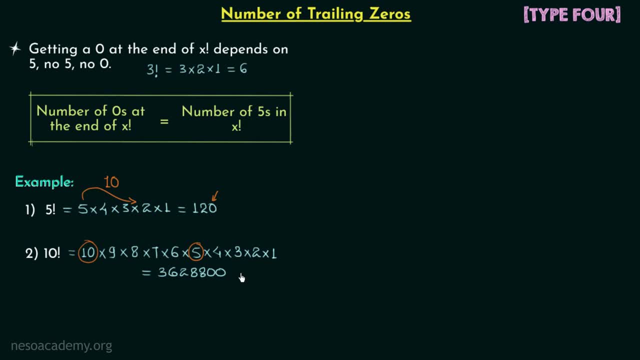 So I hope you now understand how we are getting 0s at the end of a factorial because of presence of 5s in the expansion. Now we can observe one issue in this method: For 10 factorial we have this long expansion. What if we have bigger factorial? In that case, 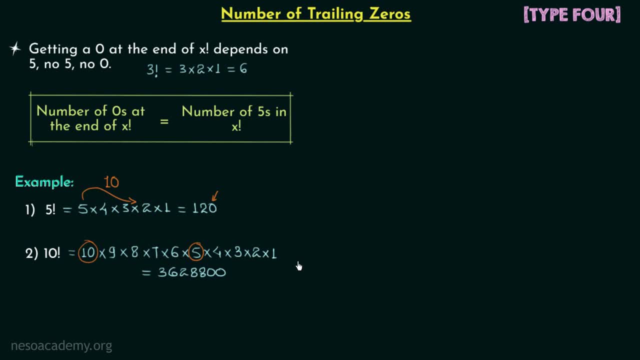 this method will become too prone to the errors. So, instead of finding the number of 0s at the end following this method, we will use this formula. We don't have to worry about the derivation of this formula. We can directly use it to find the number of 0s at the end of. 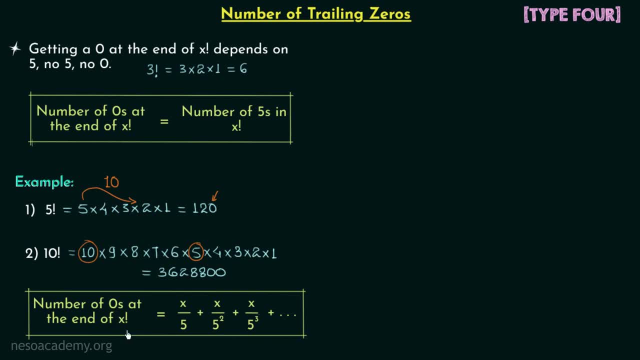 x factorial. The 0s at the end of x factorial will be equal to x over 5 plus x over 5 squared, plus x over 5 cubed, and so on, And in this we will be finding the integral sum. That means: 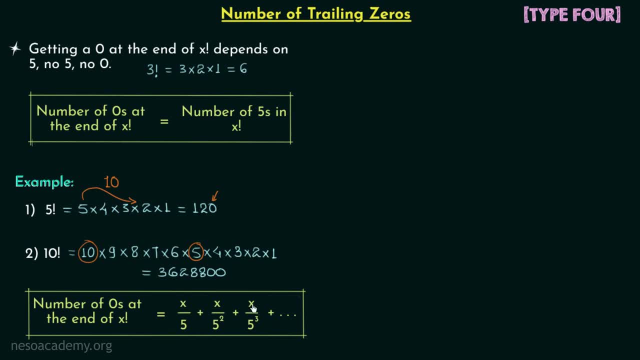 we are going to add the integer values from these divisions. Now let us solve one example problem. to apply this formula In example number 1, we need to find the number of 0s at the end of 5 factorial. We know, at the 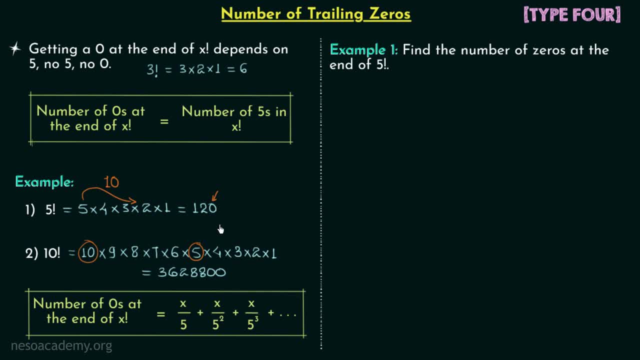 end of 5 factorial, we have one single 0. So let us check if this formula gives us the same answer. So the number of 0s at the end of 5 factorial is equal to 5 divided by 5 plus 5 divided by 5 squared plus so on. When you compare, 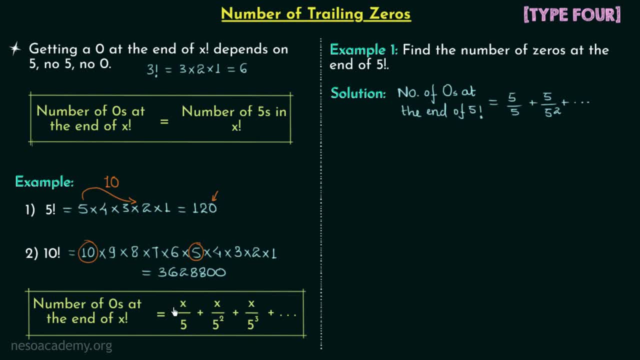 5 factorial with x factorial you will find here, in place of x we will have 5.. And then we will divide 5 by 5, raised to power 1 plus 5, divided by 5 raised to power 2 plus so on. 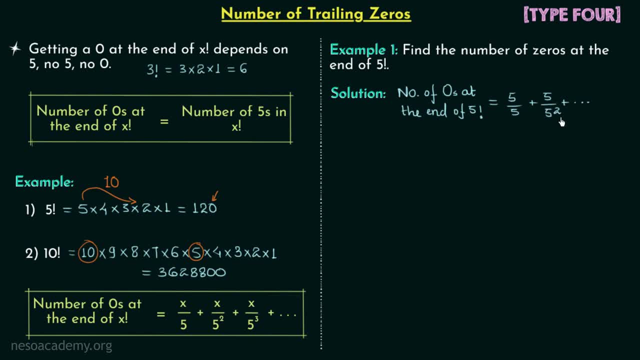 I stopped at 5 divided by 5 squared, because from this division we will get the integer part equal to 0. And similarly, all the upcoming divisions will give the integer part equal to 0. Now let us solve this. 5, when divided by 5, will give us 1.. 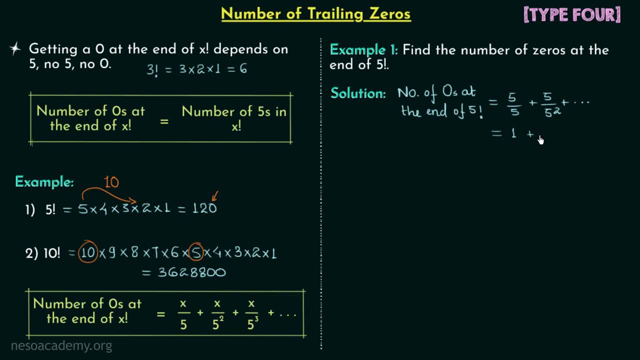 5 when divided by 25 will give us 0.2., And we will only note down the integer part. So in this way we are getting 1 as the number of 0 at the end of 5, factorial, And the same answer we got here as: 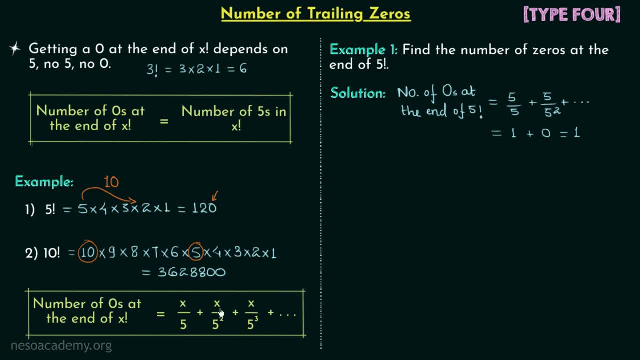 well, So from now on, we are going to use this formula to find out the number of trailing 0s or the number of 0s at the end of a given factorial. Let us now move on to example number 2.. 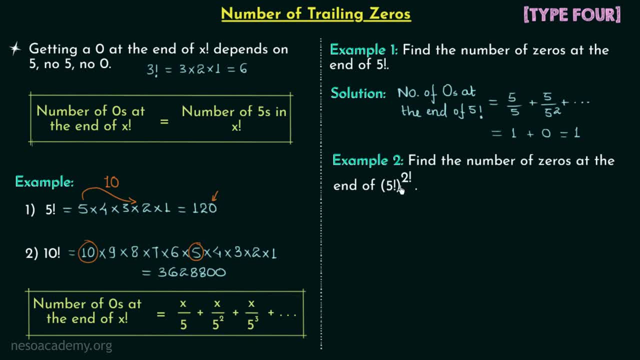 Find the number of 0s at the end of 5 factorial, Raise to power 2 factorial. So here we have something different. We have 5 factorial And then the power of 5 factorial is 2 factorial. We will first see the general. 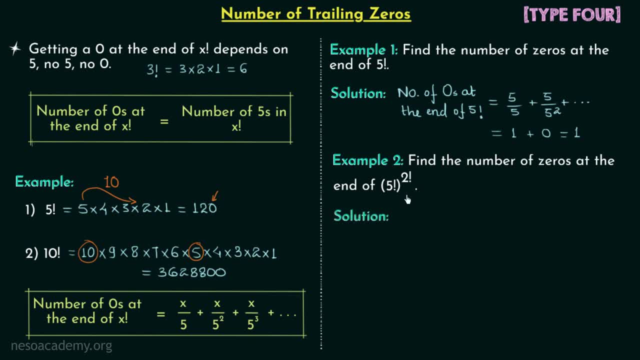 formula to solve this kind of questions. Let's say 5 factorial is x factorial and 2 factorial is y factorial. So x factorial raised to power, y factorial. We want to find out the number of 0s at the end of this. The formula is: number of 0s at the end of. 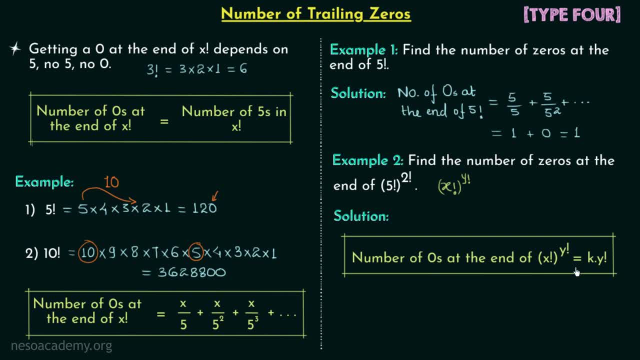 x factorial raised to power. y factorial is equal to k multiplied to y factorial. We know y factorial. It will be here. What about k? K is the number of 0s at the end of x factorial. So we first need to find out the number of zeros.